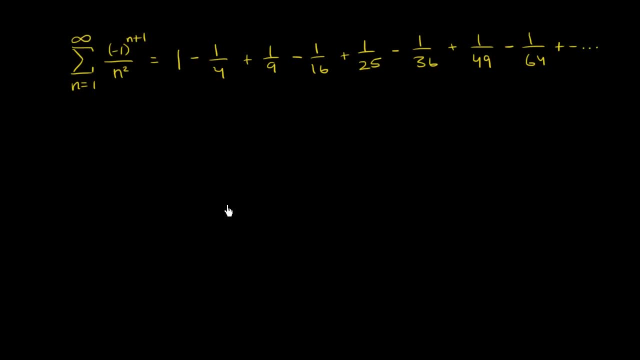 Now we know from previous tests, in fact, the alternating series test. this satisfies the constraints of the alternating series test and we're able to show that it converges. What we're doing now is actually trying to estimate what things converge to. 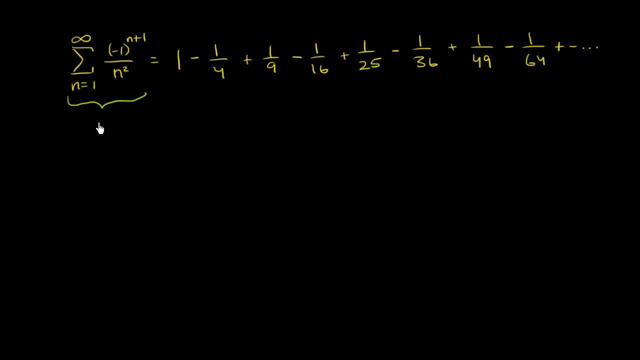 So we want to converge, so we're not converging. we want to estimate what this value s is, and we're gonna do that by doing a finite number of calculations, by not having to add this entire thing together. And so let's estimate it by taking 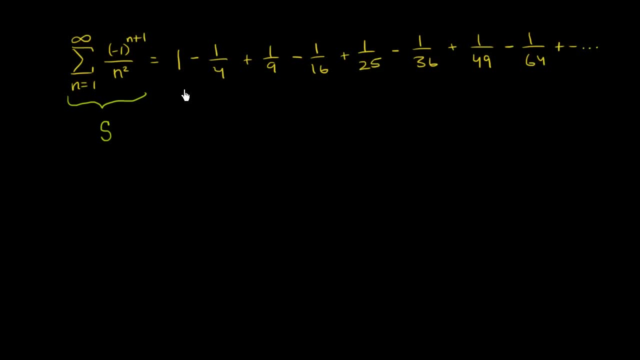 let's say, the partial sum of the first four terms. So let's take these four terms right over here and let's call that. so that's gonna be s sub four, and then you're gonna have a remainder which is gonna be everything else. 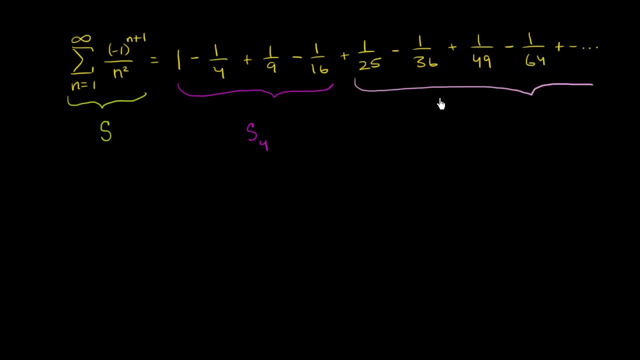 So all of this other stuff, I don't want even the brackets to end. that's going to be your remainder, the remainder to get to your actual sum or whatever's left over when you just take the first four terms. So this is from the fifth term all the way to infinity. 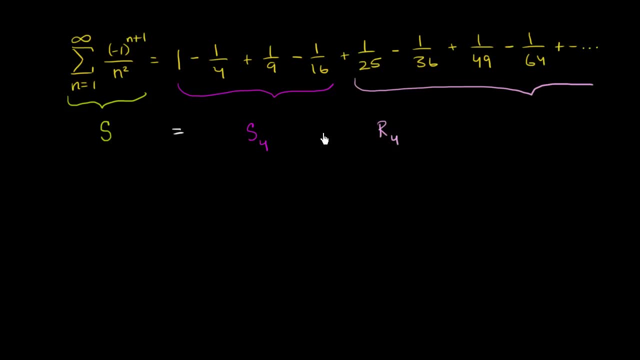 And we've seen this before. so the actual sum is going to be equal to this partial sum plus this remainder. Well, we can calculate this. this is going to be. let's see The denominator here we see, nine times 16 is 144,. 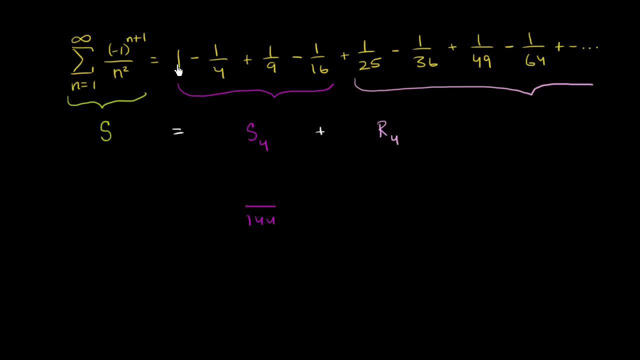 so it's gonna be 144, and then that's gonna be 144 minus 36 over 144,, plus 16 over 144, minus nine over 144,. let's see that is 144, negative 36 plus 16 is negative minus 20,. 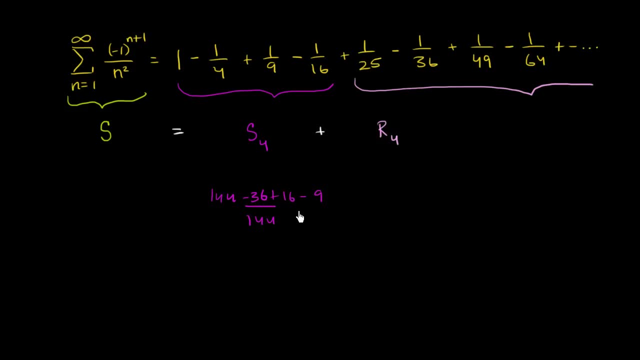 so it's 124 minus nine is 115. So this is all going to be equal to 115 over 144, I didn't even need a calculator to figure that out- plus some remainder, Plus some remainder, And so if we could figure out some bounds. 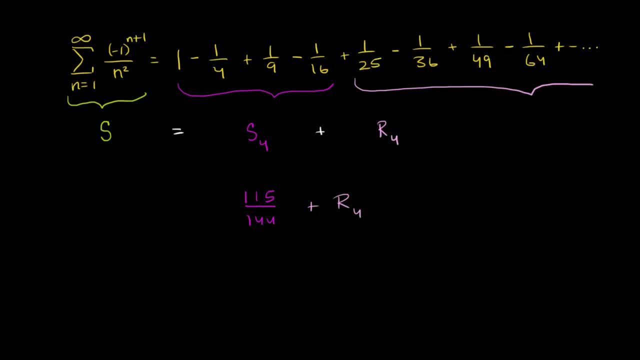 on this remainder, we will figure out the bounds on our actual, on our actual sum. We'll be able to figure out, well, how far is this away from this right over here, And there's two ways to think about it. so let's look at it. 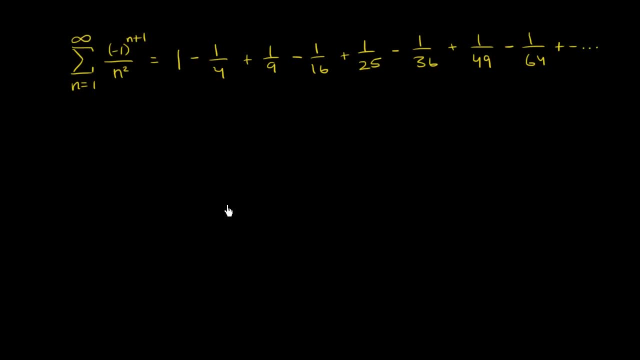 Now we know from previous tests, in fact, the alternating series test. this satisfies the constraints of the alternating series test and we're able to show that it converges. What we're doing now is actually trying to estimate what things converge to. 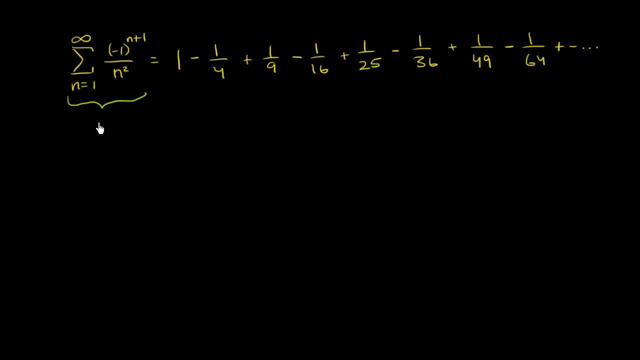 So we want to converge, so we're not converging. we want to estimate what this value s is, and we're gonna do that by doing a finite number of calculations, by not having to add this entire thing together. And so let's estimate it by taking 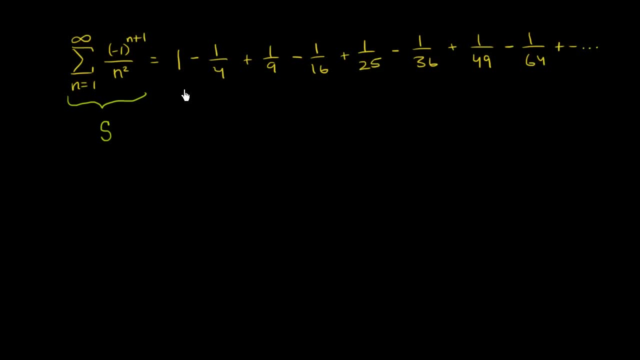 let's say, the partial sum of the first four terms. So let's take these four terms right over here and let's call that. so that's gonna be s sub four, and then you're gonna have a remainder which is gonna be everything else. 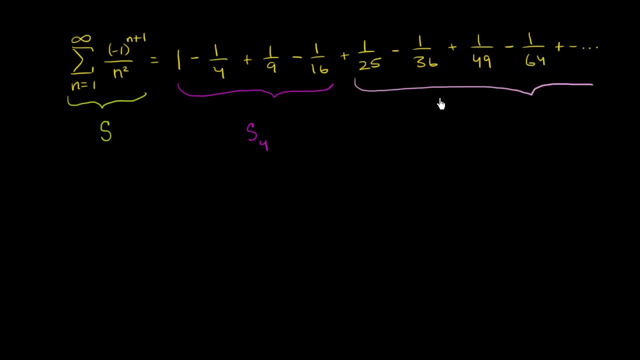 So all of this other stuff, I don't want even the brackets to end. that's going to be your remainder, The remainder to get to your actual sum or whatever's left over when you just take the first four terms. So this is from the fifth term all the way to infinity. 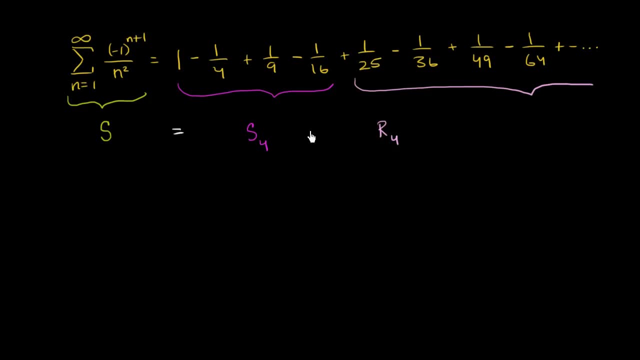 And we've seen this before. so the actual sum is going to be equal to this partial sum plus this remainder. Well, we can calculate this. this is going to be. let's see The denominator here. we'll see nine times 16 is 144.. 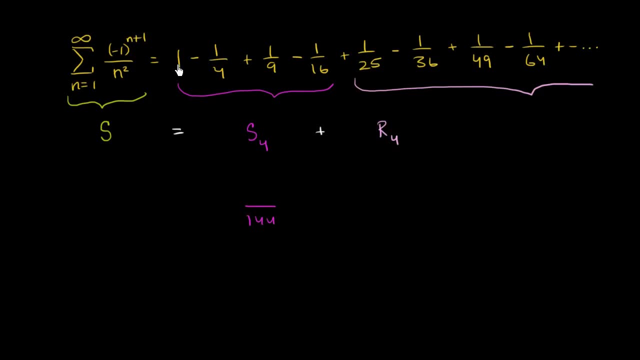 So it's gonna be 144, and then that's gonna be 144 minus 36 over 144,, plus 16 over 144, minus nine over 144, let's see that is 144, negative. 36 plus 16 is negative minus 20.. 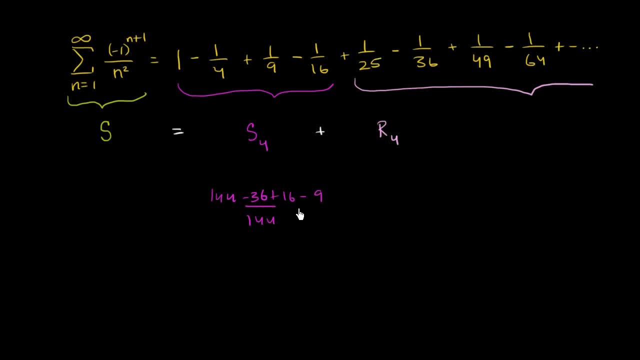 So it's 124 minus nine is 115. So this is all going to be equal to 115 over 144, I didn't even need to calculate or figure that out- plus some remainder, Plus some remainder, And so if we could figure out some bounds, 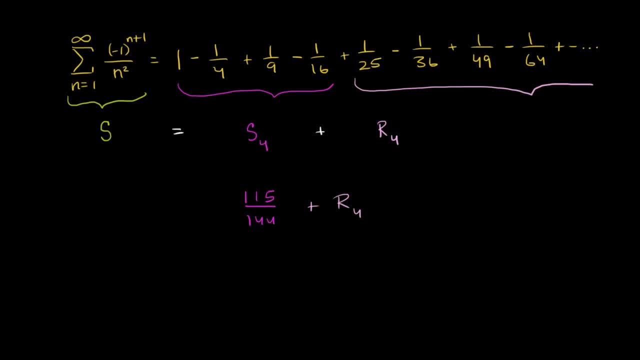 on this remainder, we will figure out the bounds on our actual, on our actual sum. We'll be able to figure out, well, how far is this away from this right over here, And there's two ways to think about it. So let's, let's, let's look at it. 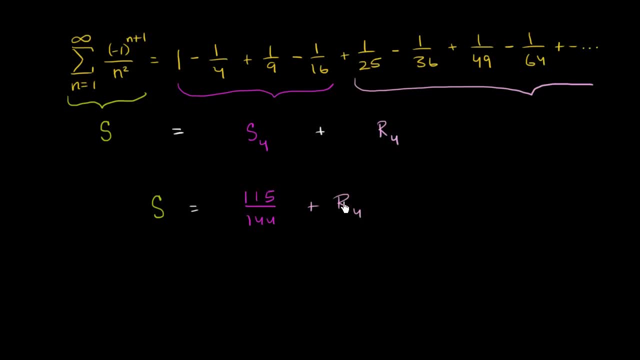 So the the first thing I wanna see is I wanna show you that this remainder right over here is definitely going to be positive, And I actually encourage you to pause the video and see if you can prove to yourself that this remainder over here is definitely. 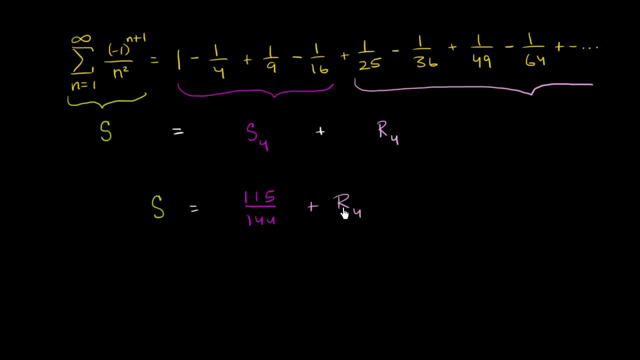 So the first thing I want to see is: I want to show you that this remainder right over here is definitely going to be positive, And I actually encourage you to pause the video and see if you can prove to yourself that this remainder over here is definitely going to be positive. 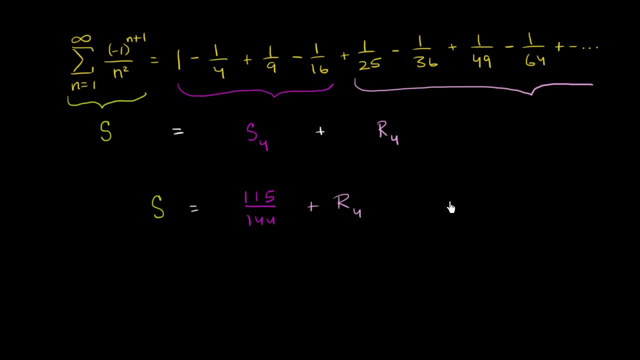 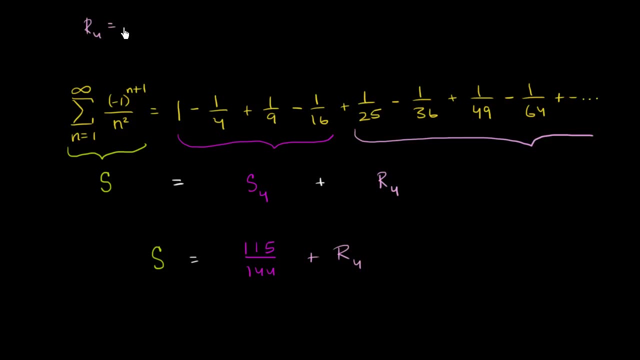 So I'm assuming you've had a go at it, Let's write the remainder down. So actually I'll just write it. actually I'll write it up here. so R sub four is one over four, one over 25, one over. actually I don't even have 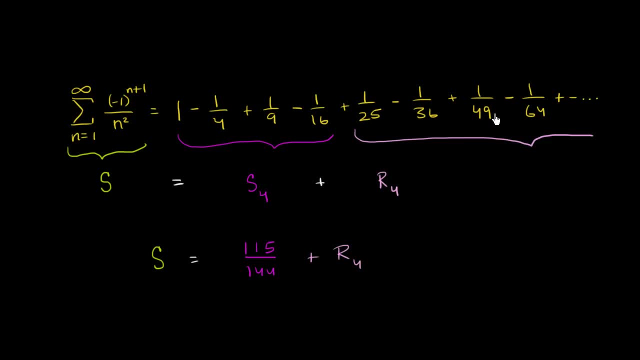 to write it separately. I can show you in just right over here that this is going to be positive. How do I show that? Well, we just pair. let's just put some parentheses in here and just pair these terms like this: So one over 25 minus one over 36.. 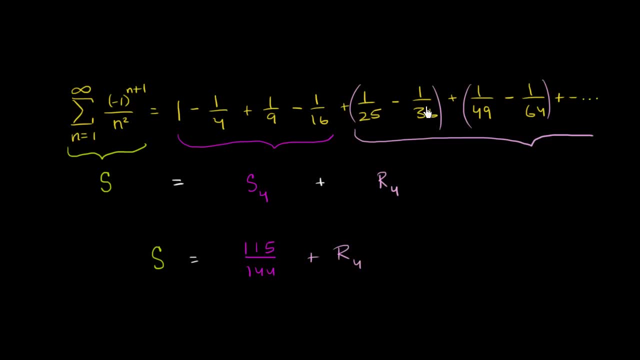 136 is less than one over 25.. This one's positive, this one's negative, So this is positive. Then you have a positive term, subtracting from that a smaller negative term, So this is going to be positive. And so, if you just pair all of these terms up, 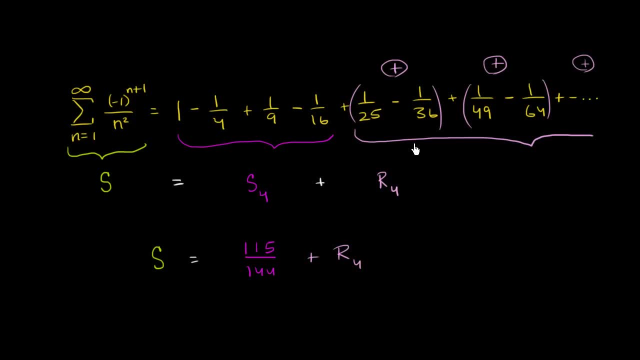 you're just going to have a whole series of positive terms. So, just like that, we have established that R sub four, or R four, we could call it- is going to be greater than zero. So R four is going to be greater than zero. 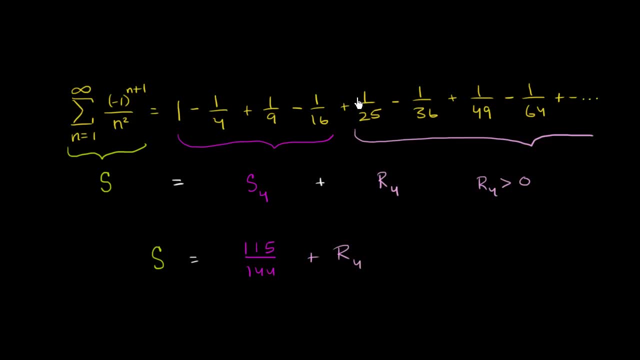 And now the other thing I want to prove is that this remainder is going to be less than the first term, that we haven't calculated, That the remainder is going to be less than one over 25.. And, once again, I encourage you to pause the video. 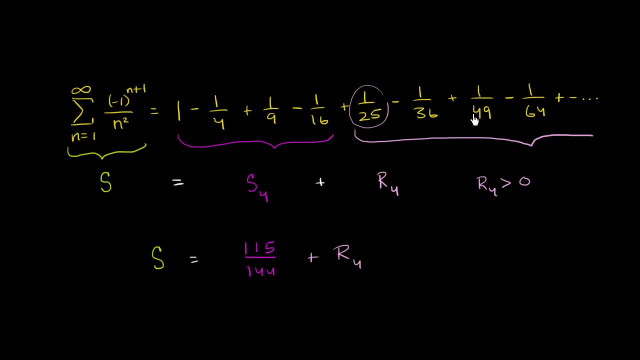 and see if you can put some parentheses here in a certain way that will convince you that this entire infinite sum here, this remainder, is going to sum up to something that's less than this first term. Once again, I'm assuming you've had a go at it. 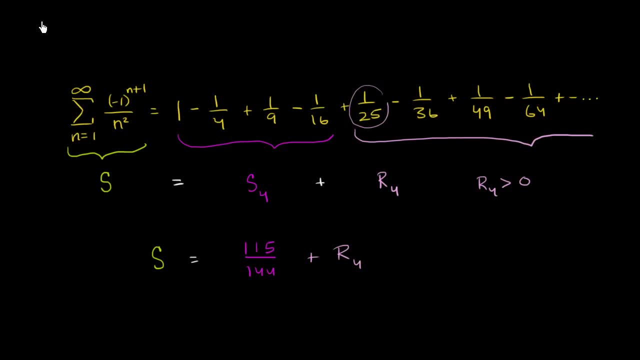 so let's just write it down. So I'll do that same pink color. So our remainder, when we take the partial sum of the first four terms, so it's one over 25, and the way I'm going to write it. 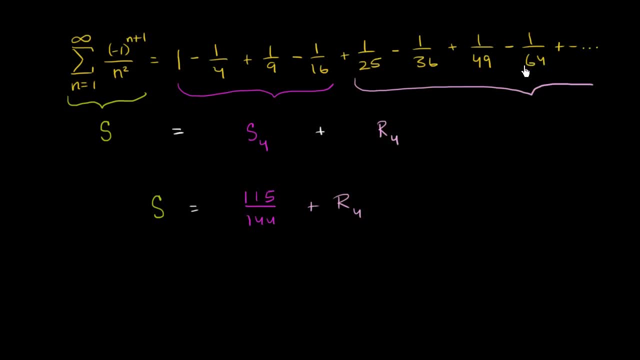 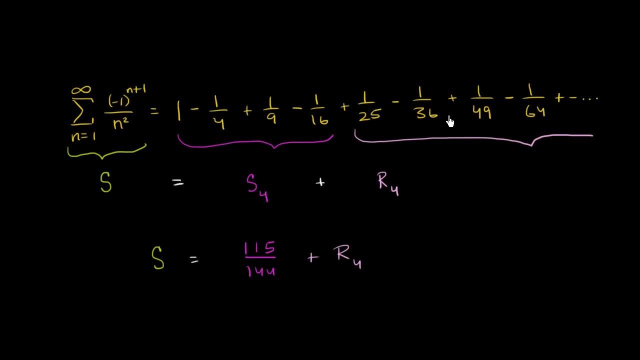 going to be positive. So I'm assuming you've had a go at it. Let's write the remainder down. So actually I'll just write it. actually I'll write it up here. So R sub four is one over. R sub four is one over. 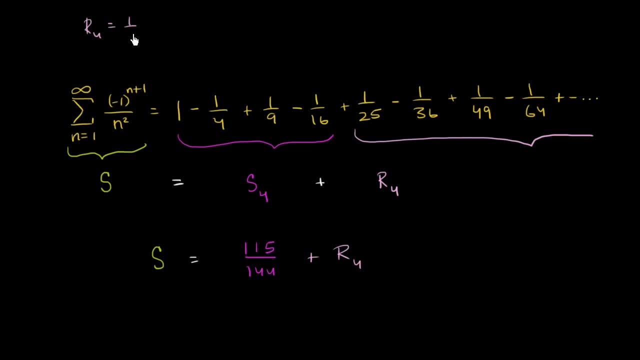 one over 25,, one over 20, actually, I don't even have to write it separately. I could show you in just right over here that this is going to be positive. How do I show that? Well, we just pair. let's just create. 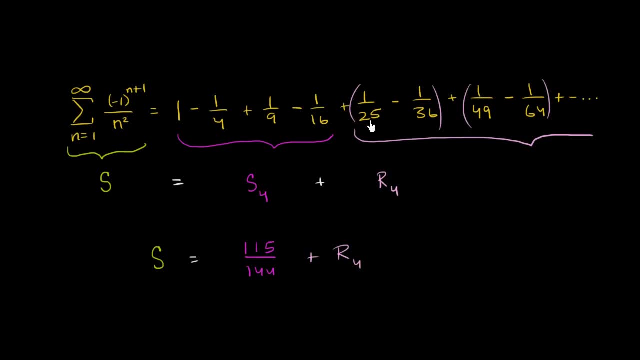 put some parentheses in here and just pair these terms like this: So one over 25 minus one over 36.. 136 is less than one over 25.. This one's positive, this one's negative. So this is positive, Then you have a positive term. 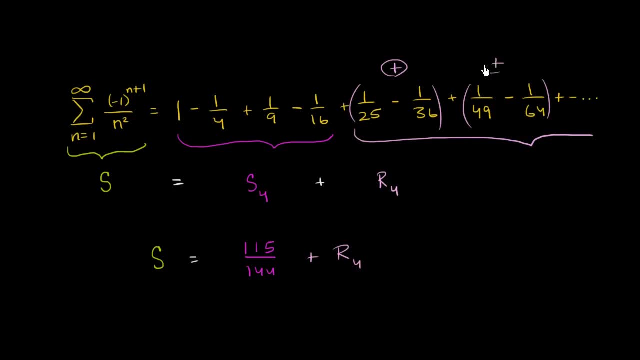 subtracting from that a smaller negative term. So this is going to be positive. And so if you just pair all of these terms up, you're just going to have a whole series of positive terms. So just like that, we have established that R sub four, or R four we could call it. 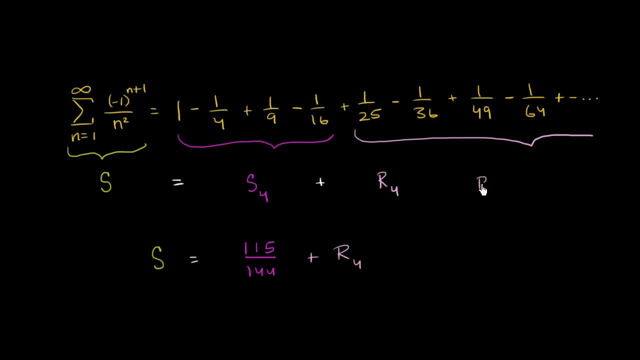 is going to be greater than zero. So R four is going to be greater than zero. And now the other thing I want to prove is that this remainder is going to be less than the first term, That we haven't calculated, That the remainder is going to be less than one over 25.. 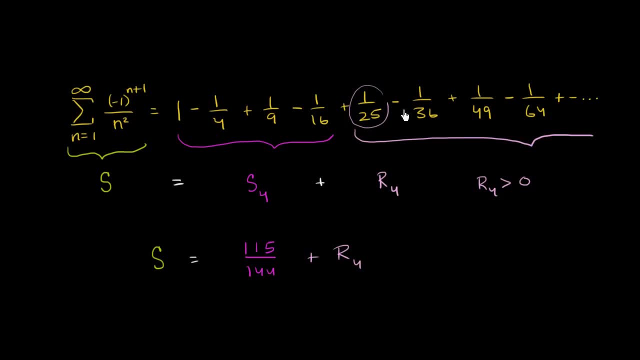 And once again I encourage you to pause the video and see if you can put some parentheses here in a certain way that will convince you that this entire infinite sum here, this remainder, is going to sum up to something that's less than this first term. 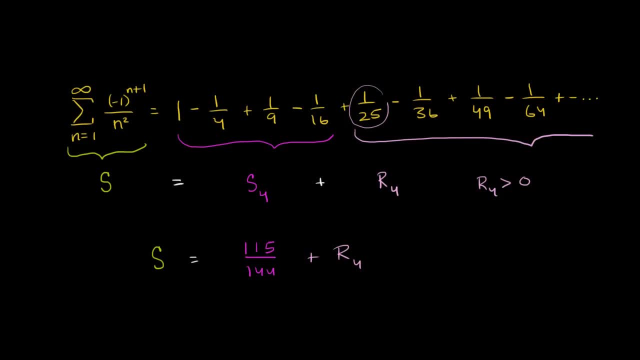 Once again, I'm assuming you've had a go at it, So let's just write it down, So I'll do that same pink color. So our remainder when we take the partial sum of the first four terms, so it's one over 25.. 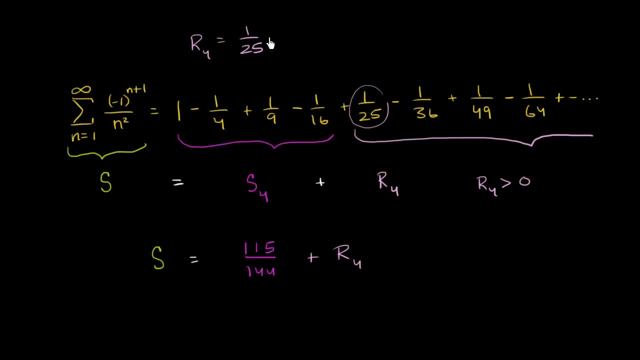 And the way I'm going to write it: instead of writing minus one over 36, I'm going to write minus. I'm going to put the parentheses now between the second, around the second and third terms. So this is going to be one over 36 minus one over 49.. 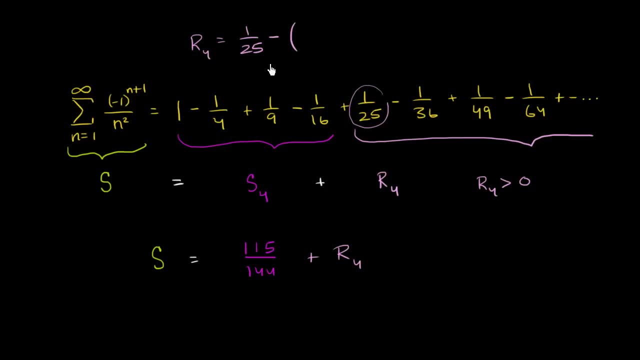 instead of writing minus one over 36, I'm going to write minus. I'm going to put the parentheses now around the second and third terms. So this is going to be one over 36 minus one over 49. And then we're going to have minus one over 64, minus. 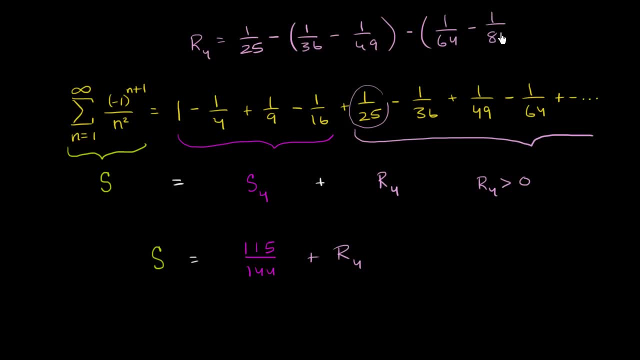 actually, the next term is going to be one over nine squared one over 81.. And then minus, and we keep going like that, on and on, and on, on and on and on forever. Now notice what happens. This term right over here is positive. 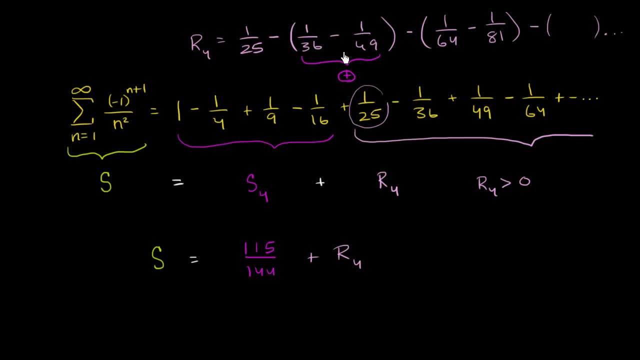 We have a smaller number being subtracted from a larger number. This term right over here is positive, So we're starting with 125, and then we're subtracting a bunch of positive things from it, So this thing has to be less than one over 25.. 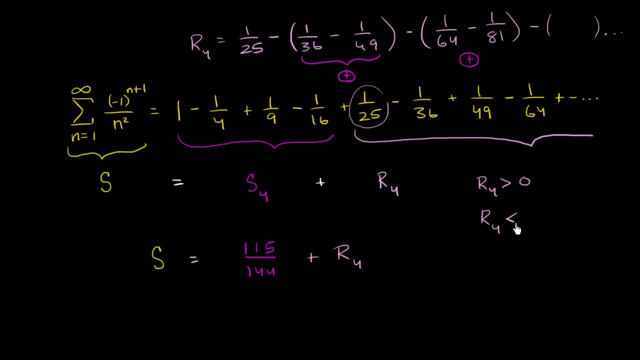 So R sub four is going to be less than one over 25.. Or we could even write that as R sub four is less than 0.04, 0.04.. Same thing as one over 25.. And actually this logic right over here. 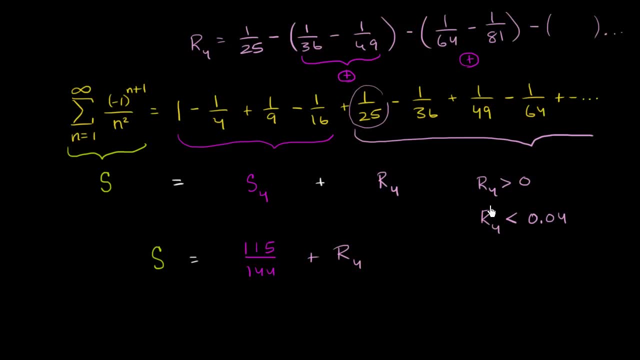 is the basis for the proof of the alternating series test. This. probably this should make you feel pretty good that, hey look, this thing is going to be greater than zero and you could, and it's increasing the more terms that you add to it. 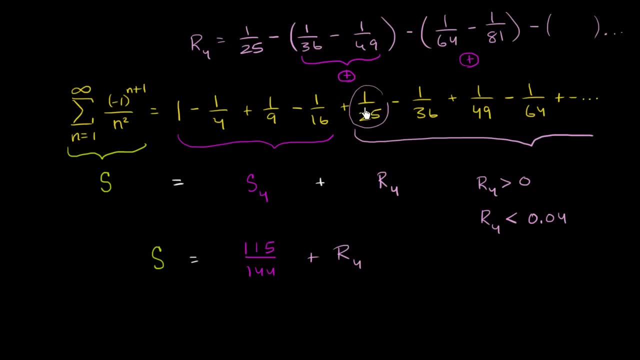 But it's bounded from above. It's bounded from above at one over 25, which is a pretty good sense that, hey, this thing is going to converge. But that's not what we're going to concern ourselves with here. Here we just care about this range. 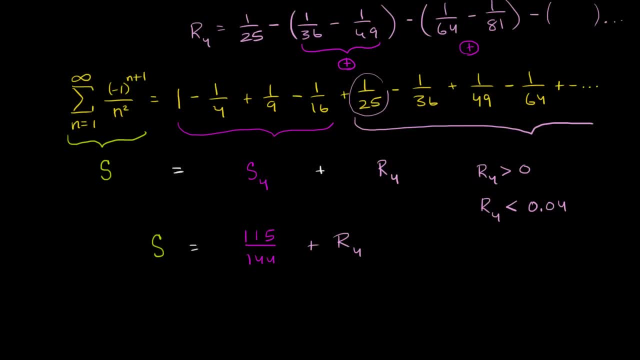 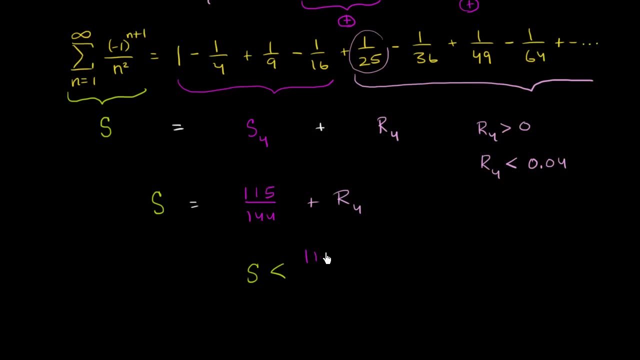 The sum is the sum of these two things, and so the entire sum is going to be less than 115,. 115 over 144, plus the upper bound on R four, so plus 0.04, and it's going to be greater than. 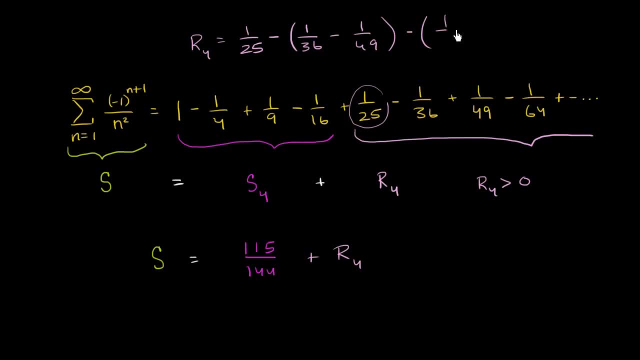 And then we're going to have minus, one over 64, minus. actually. the next term is going to be one over nine squared one over 81. And then minus, And we keep going, And we keep going like that, on, and on, and on. 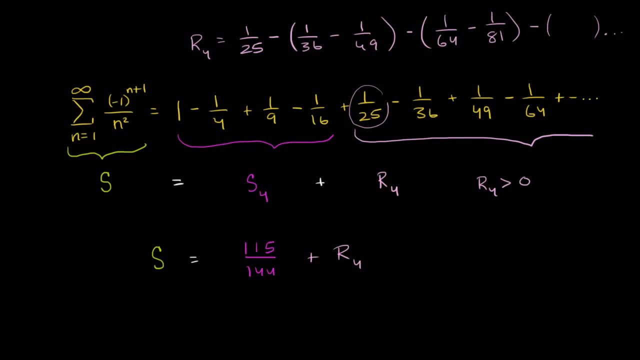 on and on and on forever. Now notice what happens. This term right over here is positive. We have a larger. we have a smaller number being subtracted from a larger number. This term right over here is positive. So we're starting with 125, and then we're subtracting. 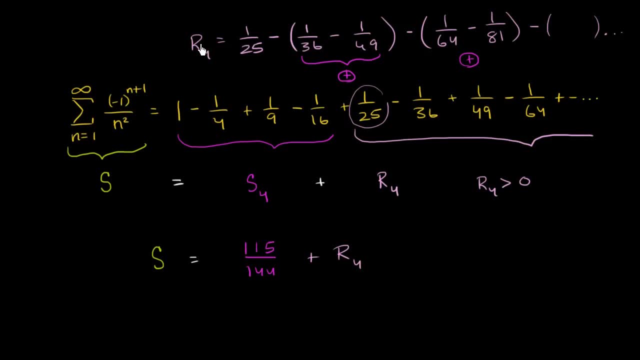 a bunch of positive things from it. So this thing has to be less than one over 25.. So r sub four is going to be less than one over 25.. Or we could even write that, as r sub four is less than 0.04, 0.04.. 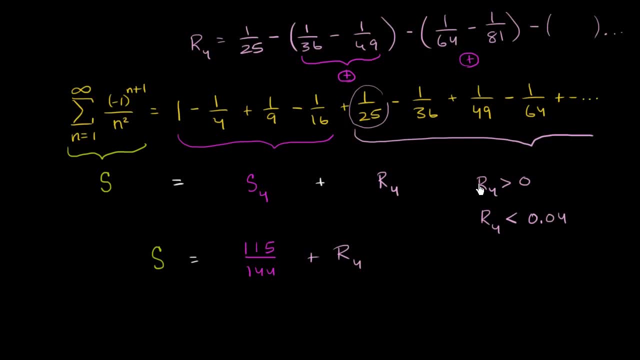 Same thing as one over 25.. And actually this logic right over here is the basis for the proof of the alternating series test. This, probably this should make you feel pretty good that hey look, this thing is going to be greater than zero. 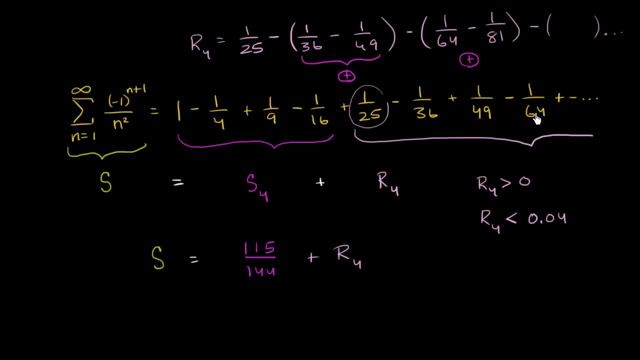 and you could, and it's increasing the more you do this and you could, and it's increasing the more you do this and you could, and it's increasing the more you do this, the more terms that you add to it. 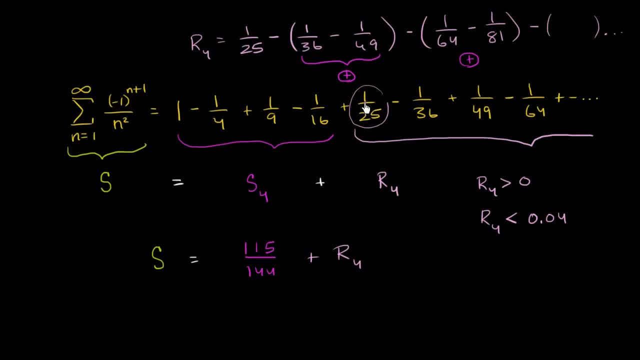 But it's bounded by. it's bounded from above. It's bounded from above at one over 25, which is a pretty good sense that, hey, this thing is gonna converge. But that's not what we're gonna concern ourselves with here. 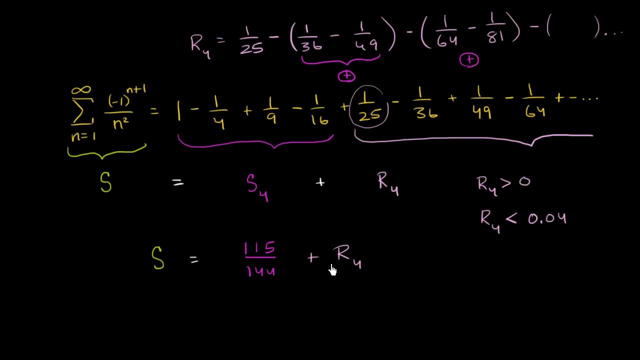 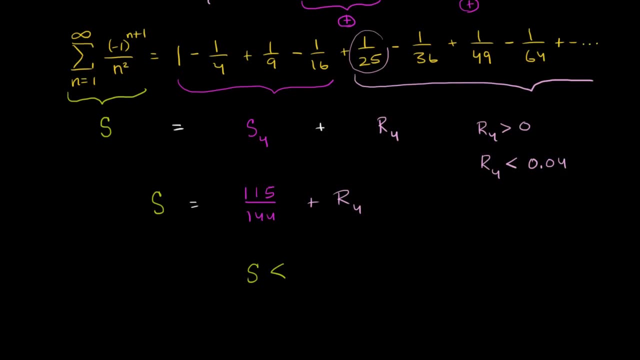 Here we just care about this range. The sum is the sum of these two things, And so the entire sum is going to be less than 115,, 115 over 144 plus the upper bound on r four, So plus 0.04, and it's going to be greater than. 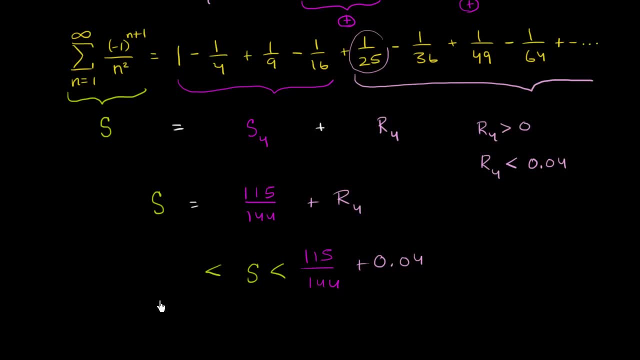 it's going to be greater than. it's going to be greater than our partial sum plus zero, because this remainder is definitely greater than zero. So you could just say it's going to be greater than our partial sum And just like that, just doing a calculation. 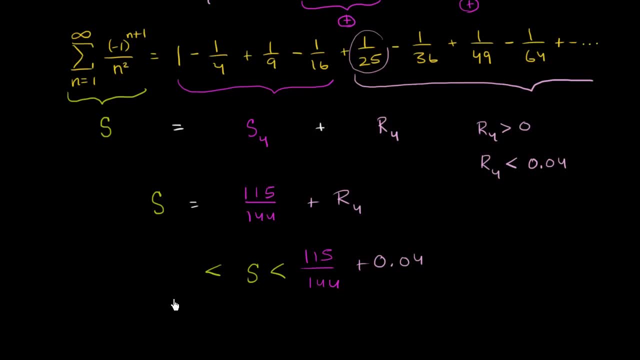 it's going to be greater than. it's going to be greater than our partial sum plus zero, Because this remainder is definitely greater than zero. So you could just say it's gonna be greater than our partial sum And just like that, just doing a calculation.